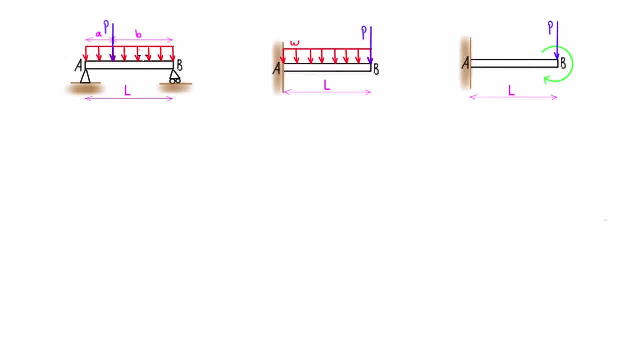 distributed load and a point load. We're actually going to work through these examples. This will be the next video, this will be the video after it and this will be the video after that, But in this video, I just want to talk about how to go about doing this. So, when we're thinking about the slope, 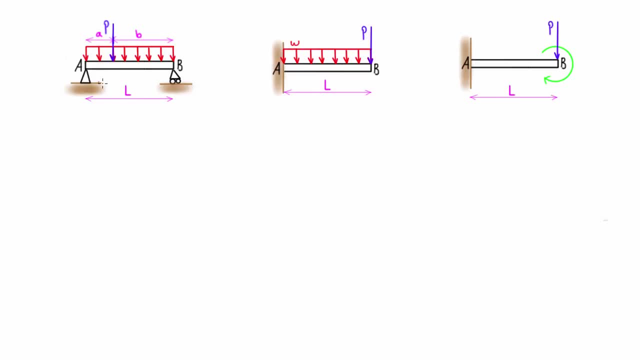 and deflection, or basically just like the actual deformed shape of one of these structures. the method of superposition tells us that that actual shape is equal to the sum of this beam when we only apply one load at a time. So, for example, this load plus this load. So basically, 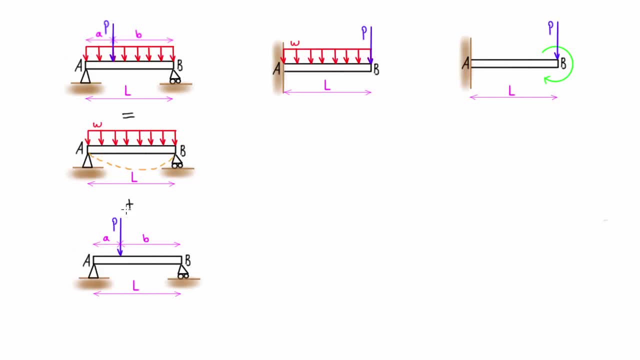 the distributed load here would cause some displacement, and this applied point load on its own would also cause some displacement, like this, And then each point would have like its own slope. And basically, if you add those together, if you add the displacement at 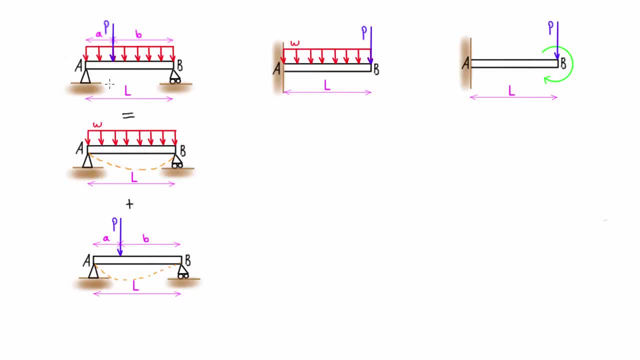 any point. or if you add the slopes at any point, that's what we're getting for the actual slope and displacement of the structure with both loads. So the same would be true for this one. If we take the actual slope and deflection of this system, then we can find it by adding up the slope and 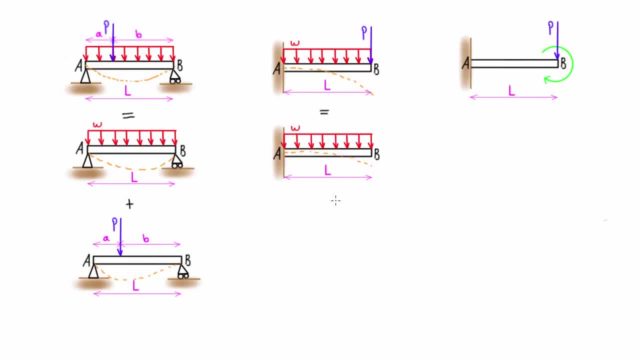 deflection caused by the distributed load and the slope, and deflection caused by just when there's a point load. And then in this example too, actually the example that I've got for you guys- I didn't realize I've got this switched here- The one that we're going to work. 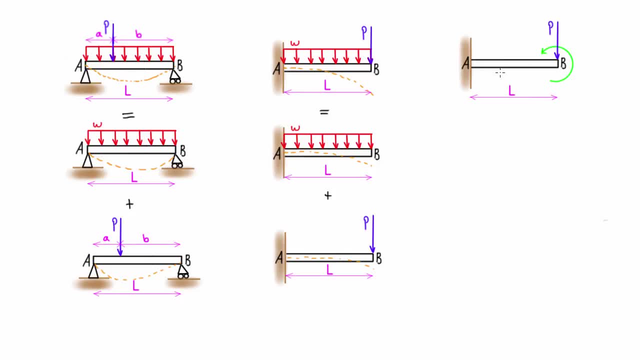 through actually has a moment like this. So the deflection of this double kind of loaded structure is going to end up looking like something like this, And that is, that can be exactly calculated by the sum of the deflection caused by the point load and the deflection caused by the applied. 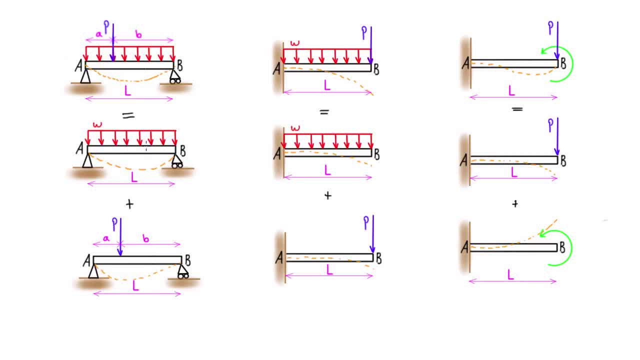 moment. So basically these just become like solving a series of easier problems where basically we're just solving statically determinate beam problems with only a single applied load. Now I want to just focus in on this part of the first problem here. If you guys have been watching my other videos, you may 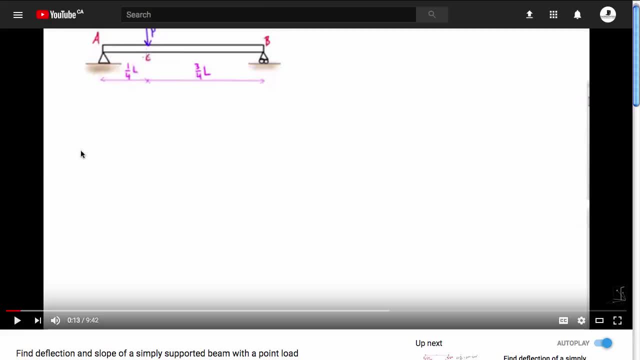 have seen me solve this problem, So this was actually the YouTube video that I did, solving that exact problem where we have a point load one quarter of the way along this span. It's called find, deflection and slope of a simply supported beam of the point load, And it's almost 10 minutes. 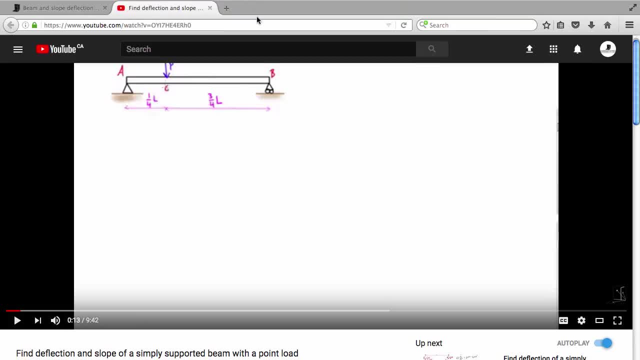 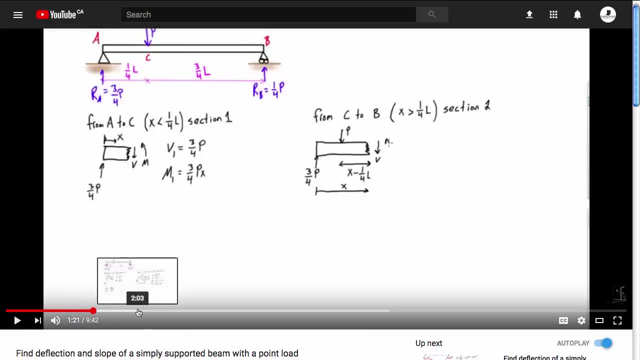 long. If you're curious, you can find the URL right there Or you can just search this by name, But this was like a 10 minute long video And as we went through, we actually we do what's called the, what's referred to as the double integration method, So we did. 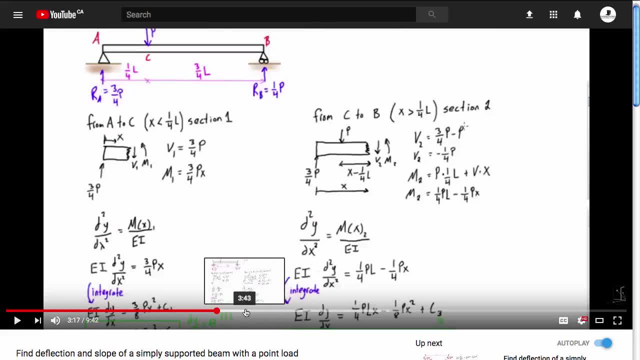 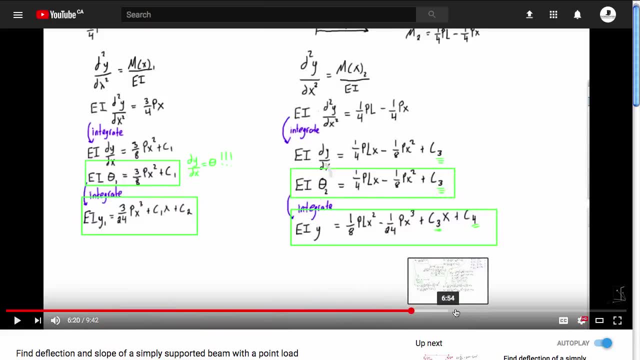 we found everything in terms of x, we integrated it twice And then we did a whole bunch of more integration stuff And if you watch this video, this might seem familiar to you, But I'm just going to skip through it So just to give you an idea of how much math was involved in this. 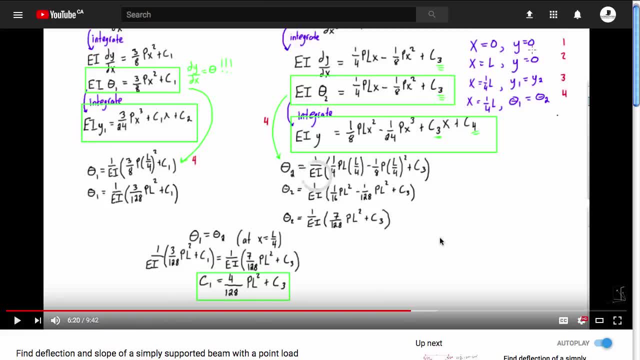 it was a. it was about a 10 minute video to watch And I'm going to skip through it So just to give you an idea of how much math was involved in this. it was a 10 minute video to watch, But most of it was. 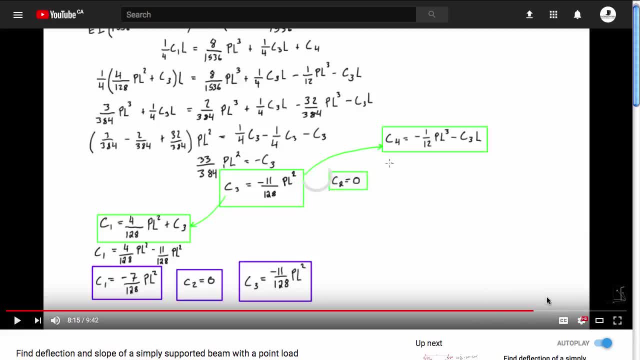 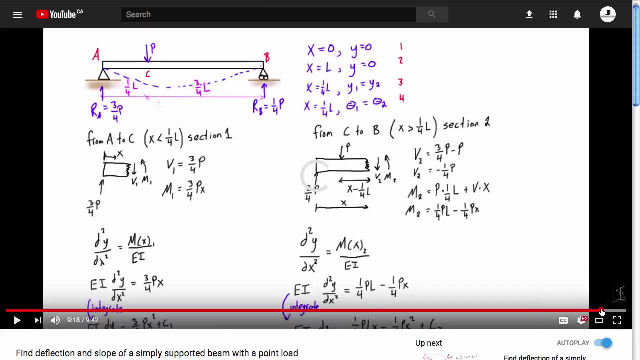 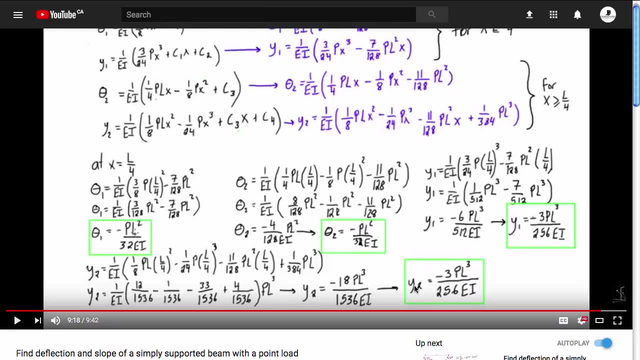 actually fast forward. it took me probably like an hour to work through this, So this is actually no easy problem. So if we get down, basically I think the end is somewhere down here. we did a whole bunch of scary math. this is like no one wants to actually do this stuff And we ended up. this was 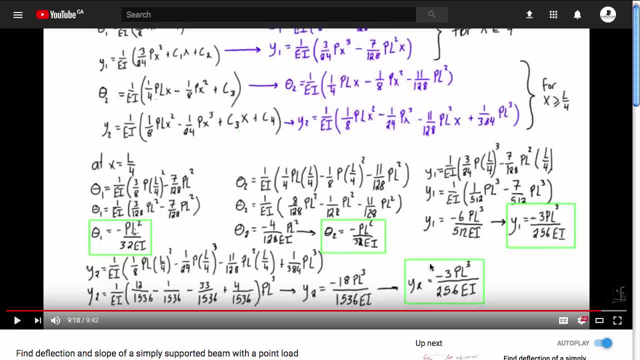 these values here. this y was our displacement at that point load And these thetas here was our angle at that point load. So crazy amounts of math just to get to there. So what I'm going to suggest that you do instead and how we're going to work through. 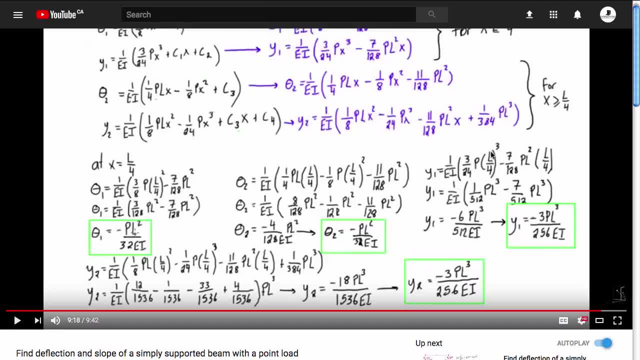 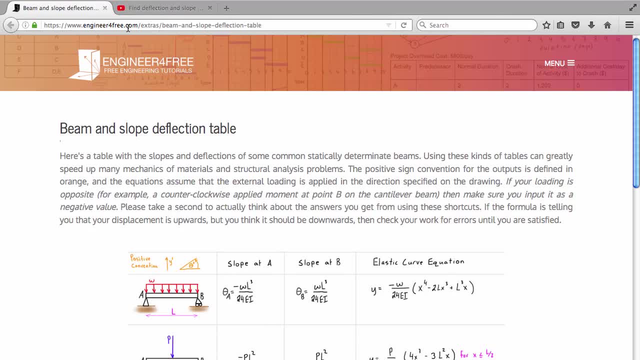 these next three problems using the method of superposition is we're going to use a table And I got that for you guys right here, So you can find this table on the website engineerforfreecom slash- all this stuff. That's the URL exactly, if you want to type it in. 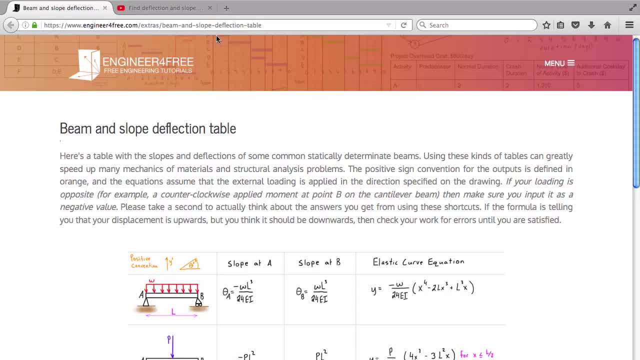 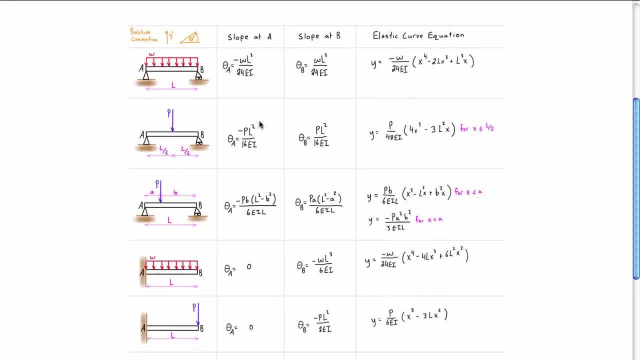 They're probably. I'm going to put a link to this in the description and maybe even put a little pop-up thing right here so you can click on that. But basically, this table here gives us for various simply supported beams. You guys can pause and read this if you want. I'm not going to read it out to. 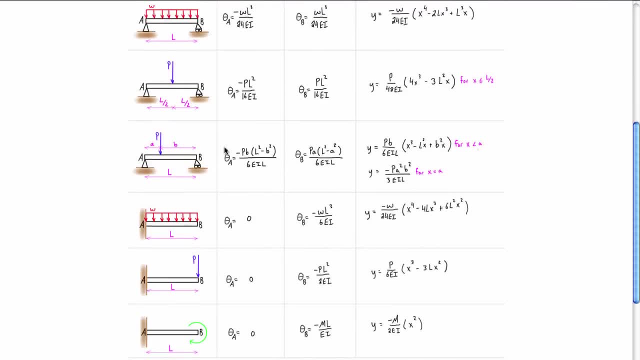 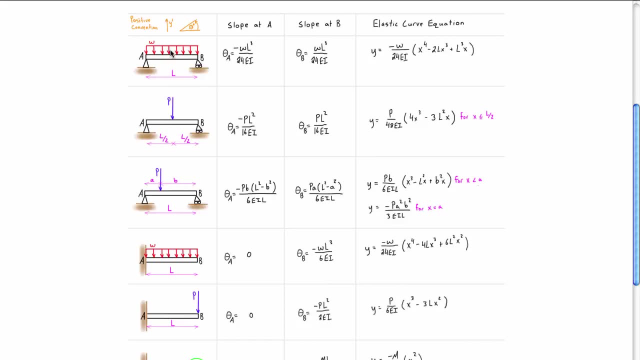 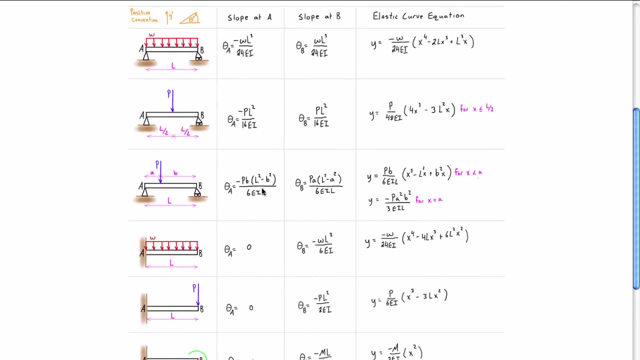 you right now, But there's some good stuff in there. So basically we have for various simply supported or so various statically determinate beams with a one type of loading, So like distributed load the whole way across, or point load, or even there's a one down here. for the moment We've got 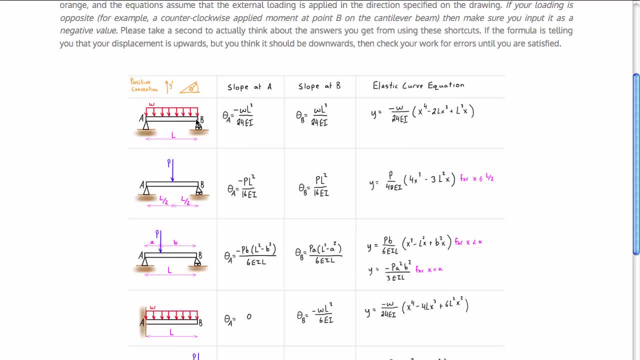 a table here. It's going to give us the slope at A, the slope at B and the elastic curve equation. There's obviously more stuff that you could put in one of these tables. You could put the max deflection or this midpoint slope or whatever. But this is going to be good enough for the next. 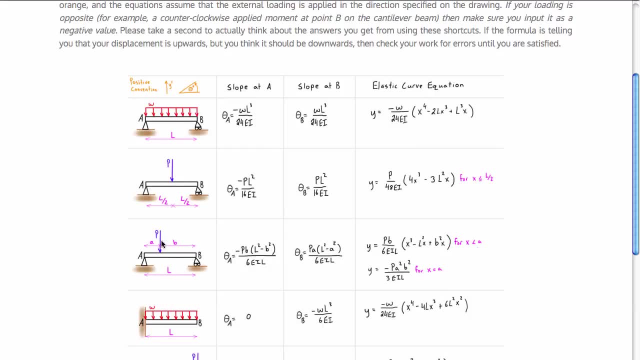 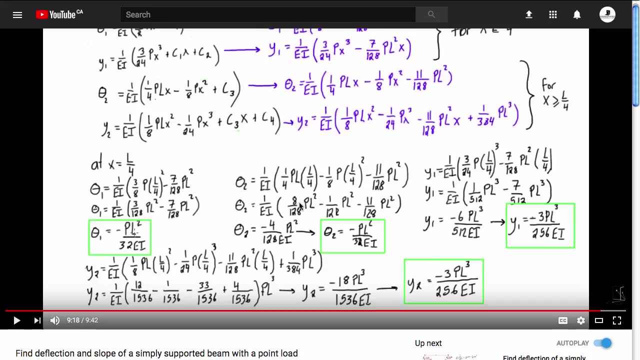 couple of videos that we're doing. So if we look at the one with a point load that's not centered in the middle, This is the exact same example that we did in in this video here. that took us like one hour to work through. 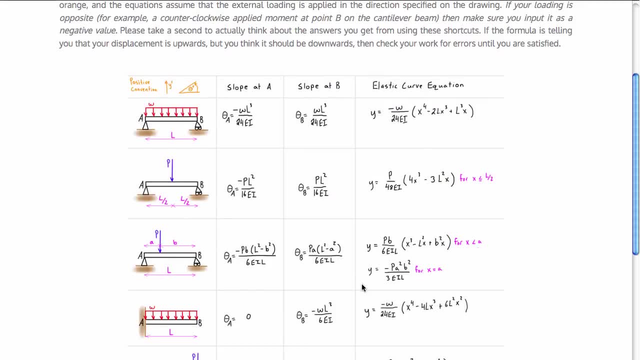 But here this is going to give us the deflection right at that point. so that's basically what we're just going to plug in and use, and this is a totally valid method and way of solving problems. you can find tables just like this in the front or back cover of any mechanics, of materials or structural analysis. 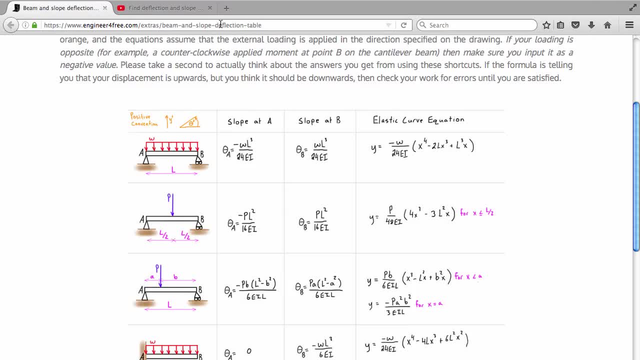 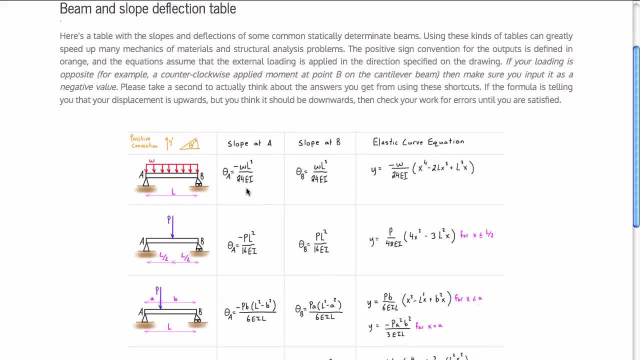 textbook or again. you can just come get this one here from that url on the website. now i do caution you guys to be super careful when you are using these that you're putting in everything correctly. for example, when you get out, when you get out values from this, outputs from these tables. if 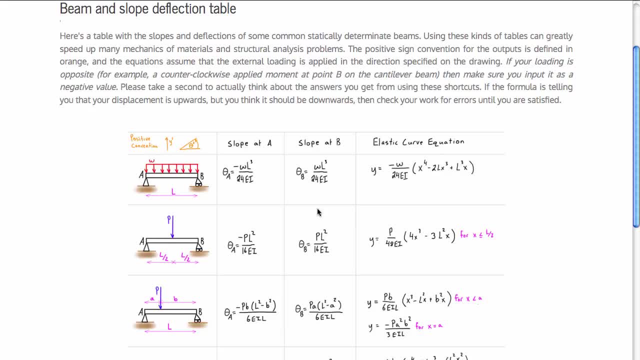 your. if your y value is positive, that's indicating a deflection in the upward direction, and if your y value is negative, that's indicating a deflection in the downward direction. and again for angles here, if you're getting a positive angle, these are in units of radians, and if it's positive, that. 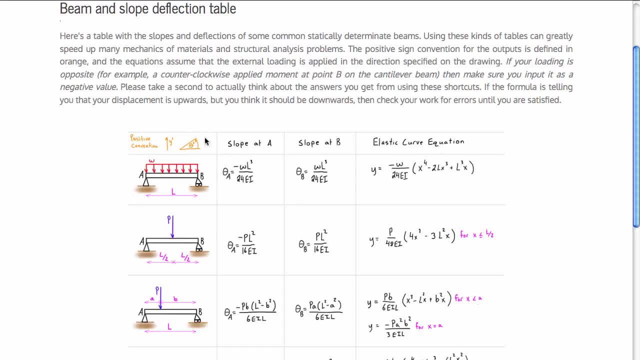 means it's kind of like clockwise up or counterclockwise up from the axis and then counterclockwise down from the axis, would be considered you a negative angle. and this positive convention is also based off of um inputting your values here, your applied load, so whether it's w, p or or m here. i forgot to label that with an m. i should. 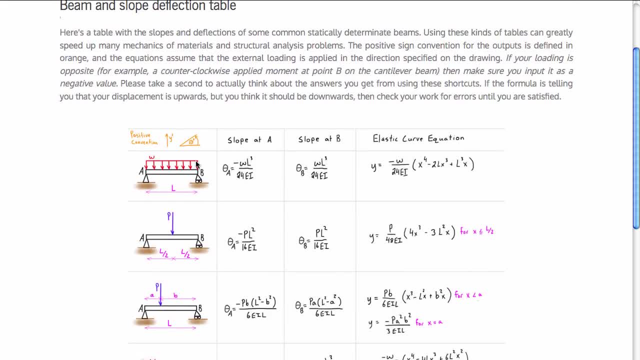 probably fix that um. but if you have, for example, like a load, like if p here is pointing up actually on the beam, then you got to put p in as a negative, otherwise it's not going to work. so i caution you to be careful when using tables, because it is really easy to get. 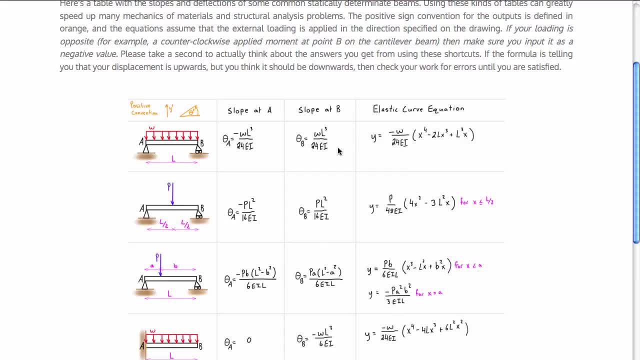 like a negative angle, and if you have a positive angle and you have a negative angle- like a negative value where you were expecting a positive one, or vice versa- you can get switched around, depending on how the the table set up. so be really cautious with that, and if you're 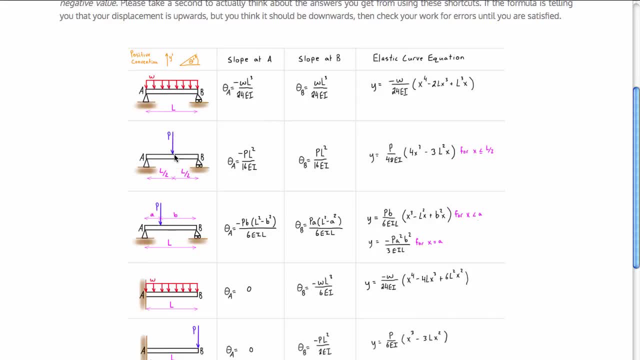 expecting something like if you have a point with pressing down and you're expecting that deflection to be downwards of the beam and you're getting some value that says it's going up again, just like: stop see if you've made a math error or something. and then, once you're satisfied with 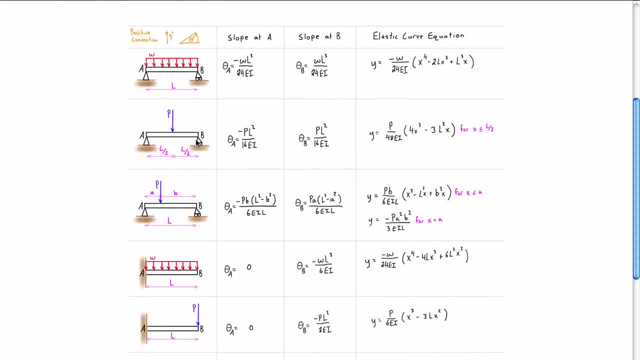 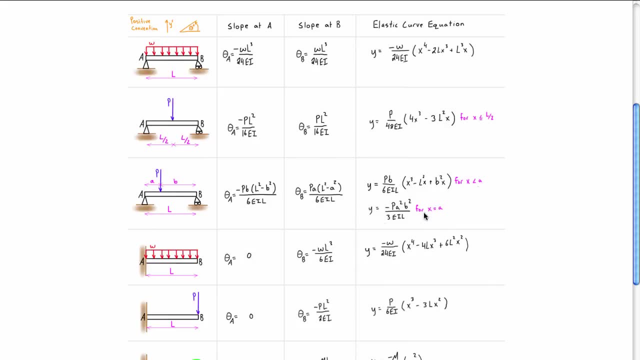 your answer, then you can. then you can proceed. so just be really careful when using tables, but they do significantly speed it up, because i bet you it's going to take us like less than a minute to type this stuff in and solve for y, whereas it took us like an hour.